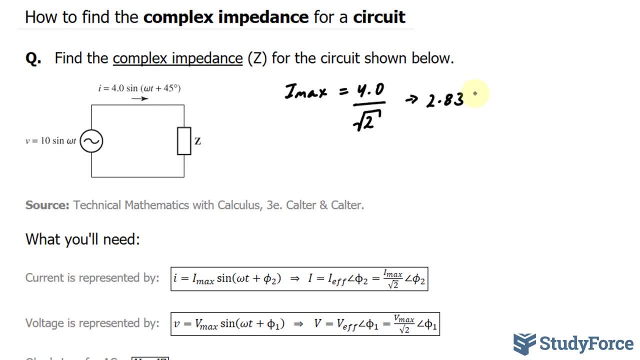 That represents my effective current And my angle is 45 degrees. So to write this down in complex polar form, I'll write down: capital I is equal to 2 decimal 8, 3, at an angle of 45 degrees. I have to do the same thing now for my voltage. 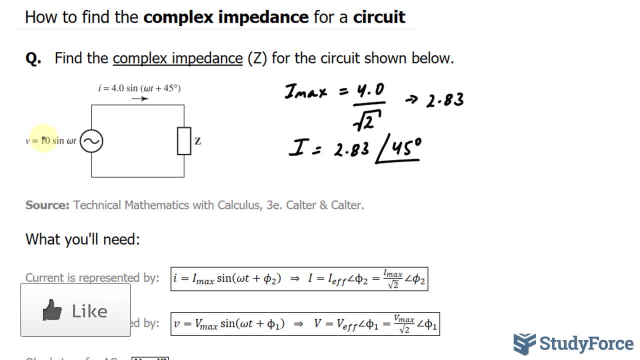 So this number 10 represents Vmax, And I can find the effective voltage by taking my Vmax, my amplitude, and dividing by the square root of 2.. So Vmax is equal to 10.. Divide that by the square root of 2.. 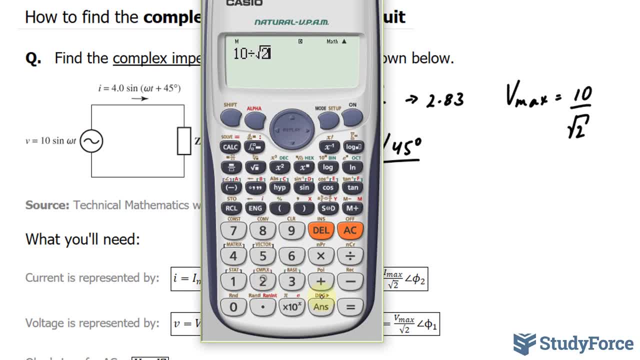 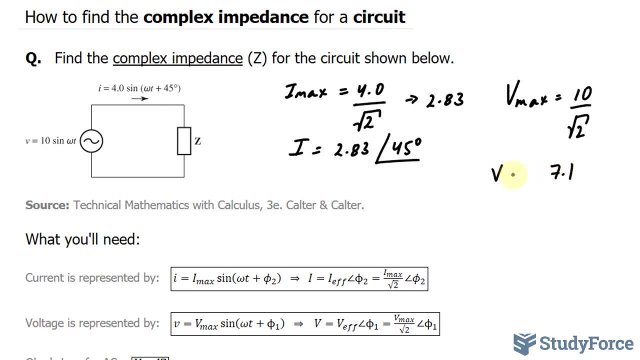 7.1.. This will represent my effective voltage 7.1 at an angle of, And no angle is provided. The phase angle here is 0.. So I'll write down 0 degrees. The question is asking for the complex impedance. 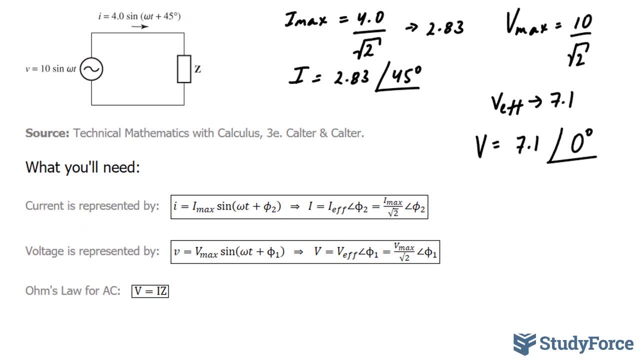 All we have to do right now is use the following relationship: Where V is equal to I, times Z, Rearranging this formula by dividing both sides by I. Take a look I end up with Z is equal to V over I. So let's go ahead and substitute what we just found earlier. 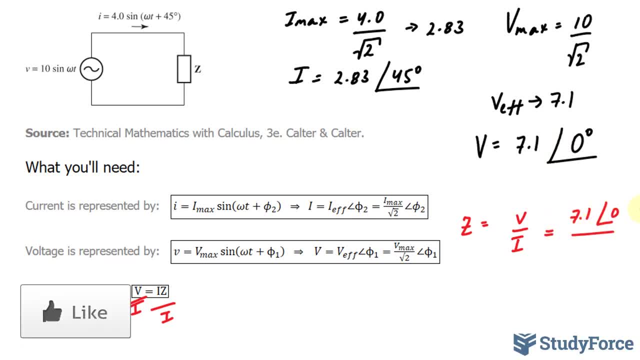 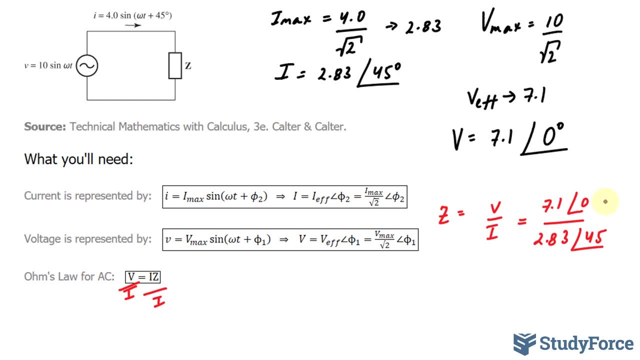 7.1 at an angle of 0, over 2.83 at an angle of 45.. We are dividing two complex polar form numbers And to do that we divide the radii 7.1.. Divided by 2.83.. 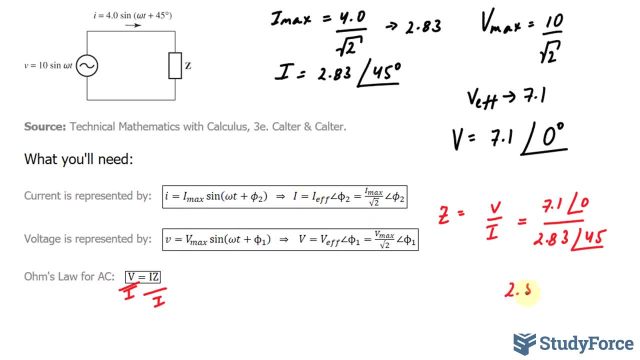 That gives me 2.50.. At an angle of 0 minus 45.. We are subtracting the two phasors, Giving us negative 45 degrees, And that right there represents the impedance In polar form for the circuit. And so there you have it. 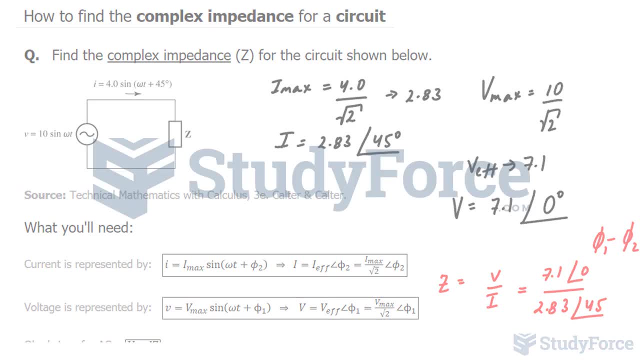 That is how to find the complex impedance for a circuit Where the modulate circumference of Z is equal to Z, like it is. check at the terminal: It shows that 0.2 radii and E is equal to 1.. So what will voy a' take for the计 alφ speakers? So I detailed that And so did I. So I gave my group two kommt-ían. That gave me the input, That give me the input, That gave me the input And that gave me the input.